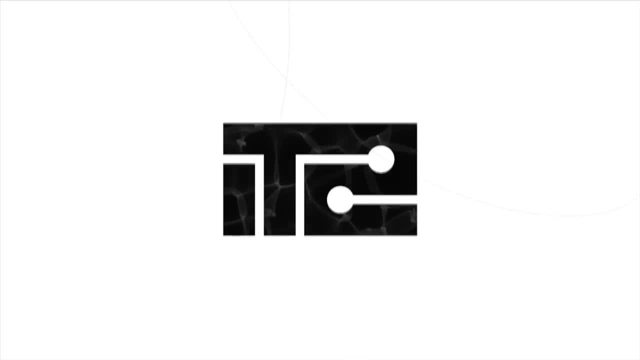 something to be learned in a couple 10 minute videos. Here's a piece of code for the Fibonacci function. Pretty beautiful. you just define the first two cases: 0 is 0,, 1 is 1, and then recursion. for the rest, Should be pretty easy to understand. 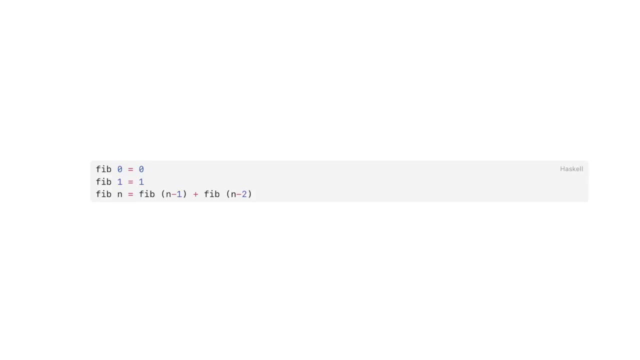 what it's doing. Here's another piece of code for sorting a list using quicksort, Although we have some weird syntax over here: p, colon xx. it's a pattern matching thing which just assigns the pivot p to the first element and xs for the rest of the list, and then we just put. 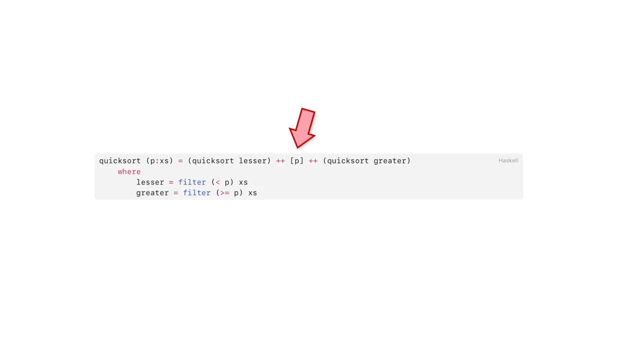 the p element in the middle and join it with the lesser and greater elements of the list, both recursively sorted. Both of them are defined at the bottom with the filter function. This is a little bit more complicated, but I'm hoping it's not too hard to understand. 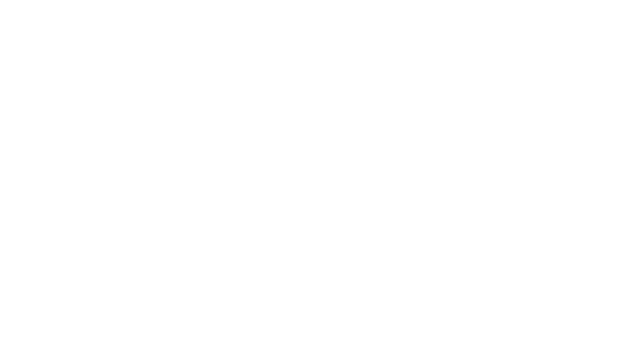 if you know what the quicksort function does in other languages, The next logical thing to do would be figuring out how to print hello world. but it's actually impossible, At least without cheating. but it's still cheating in a pretty interesting way. 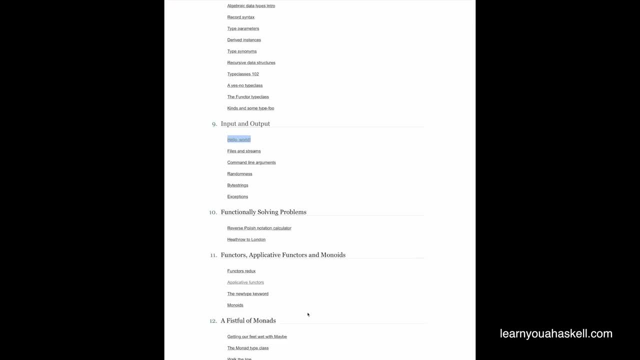 Look at this beginner Haskell book. We go through lists, strings, recursions, functions, sorting algorithms, modules, types, and then we get to printing things in chapter 9.. That's because printing is a straightforward, normal way. It's one of those things that the Haskell 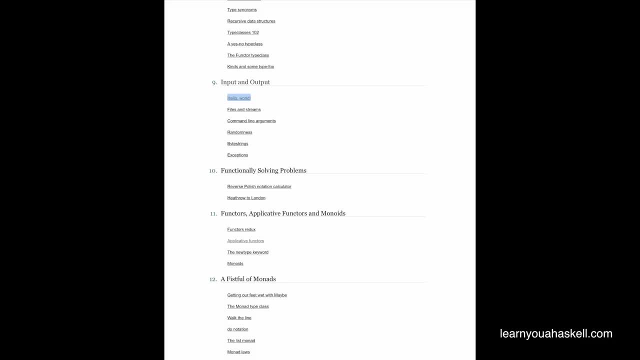 rules forbids, so it instead relies on an infamously hard to grasp concept in Haskell's design called monads. Anyway, this rule is a result from the idea of purely functional programming, and it's not just a different way of writing code compared to other languages, but a completely fundamental 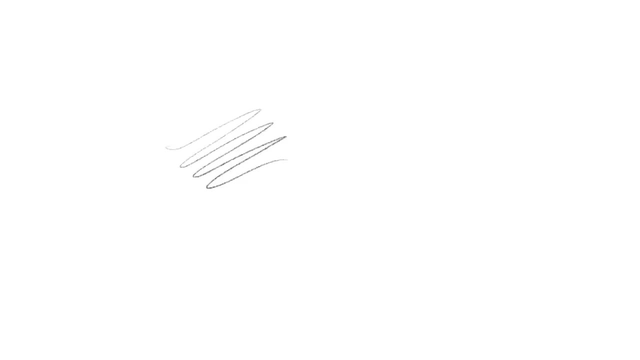 difference in computing. To explain this difference and why it's useful, we'll take a detour to some history and look at a bit of deep computer theory. So our typical style of programming goes step by step from the top of the file to the bottom. 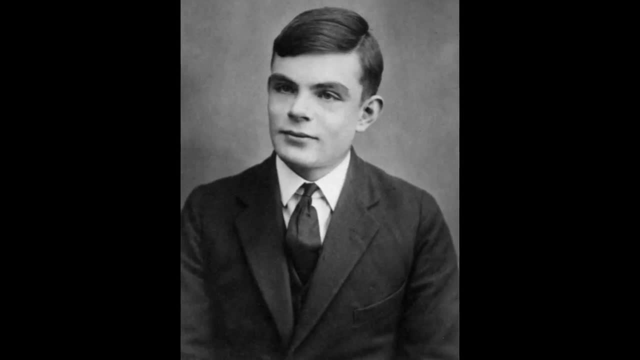 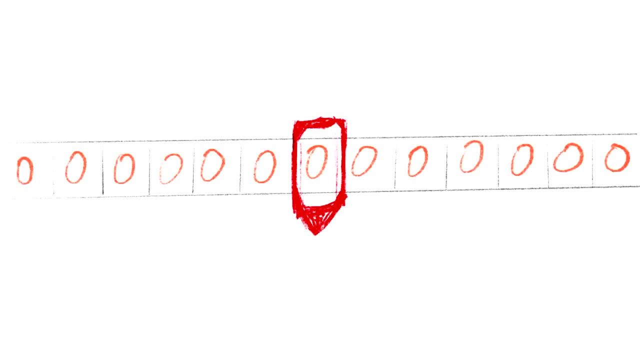 In 1936, Alan Turing, known as one of the founders of computer science, made a theoretical computer called the Turing machine. It also has a step-by-step idea of how to print a number, but it's pretty simple. The cursor can move around and change numbers and we 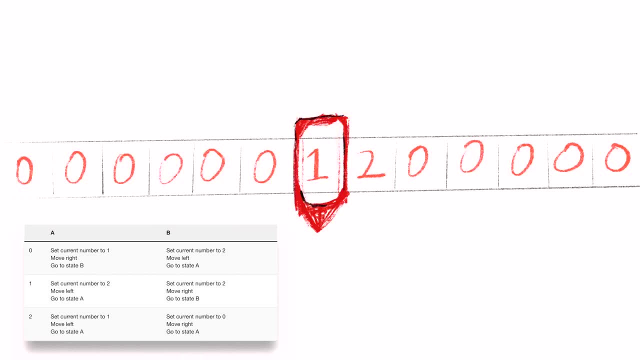 just follow a flowchart or a table to see how it moves, Depending on the number. the cursor sets the number underneath. it moves left or right and changes the state. Then each state has its own rules on what to do with the next number. and this is enough to 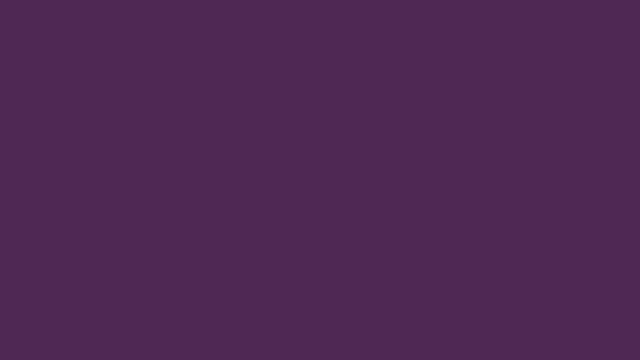 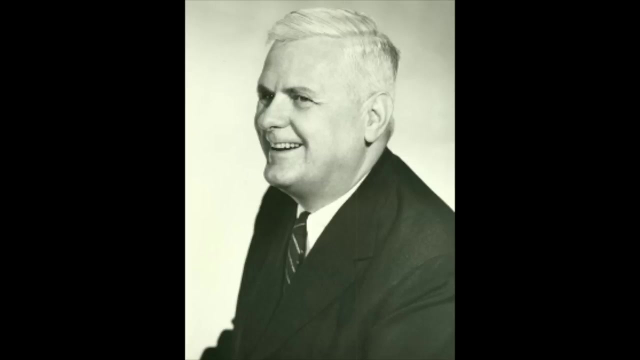 be able to compute anything that can be computed. Here's where Haskell differs. There's another, maybe simpler way of expressing calculations: lambda calculus, invented by one of Alan Turing's teachers, Alonzo Church pretty equally as well. It sounds like pretty complicated math, but the word calculus just means relating. 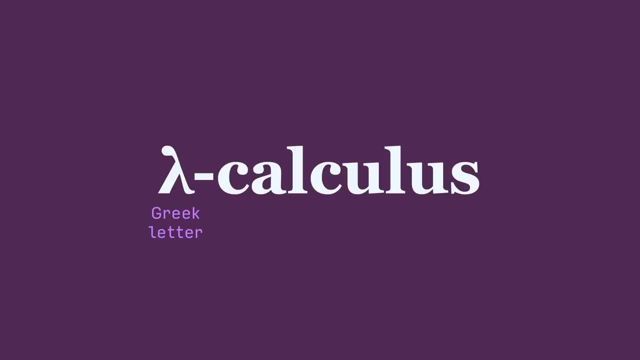 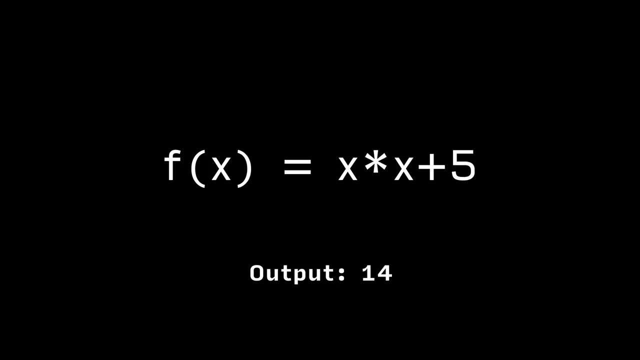 to calculations, and lambda is just a greek letter. Here all calculations are represented by math functions like fx equals x squared plus 5, and they just take an input and give an output and that's it. Your entire program is a one-line expression, like f, of g, of x. 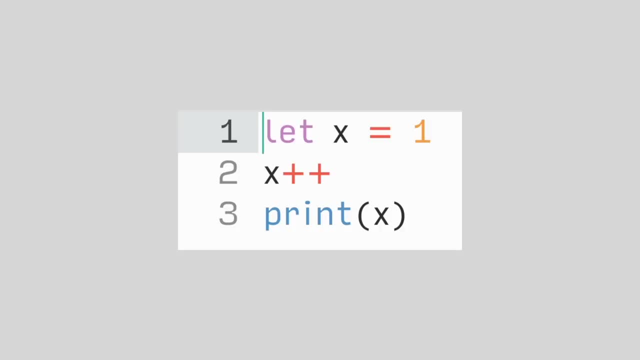 and you can run the program by evaluating the answer. There are no step-by-step commands in lambda calculus. order is only defined by what is needed to get the answer. So for example, f of g of x is the number of steps you have to do to get the answer. So for example: 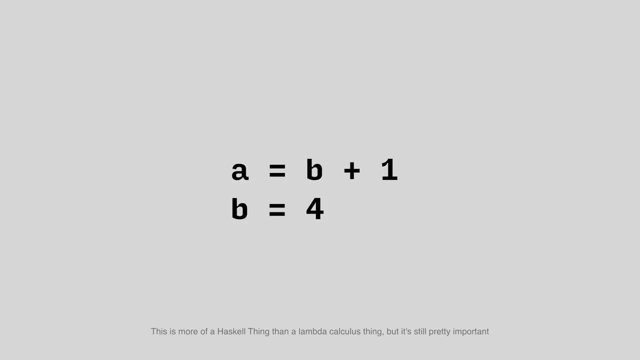 f, of g, of x is the number of steps you have to do to get the answer. So, for example, if we write, a equals to b plus 1, b equals to 4. And if you want to find a, you have to find b. 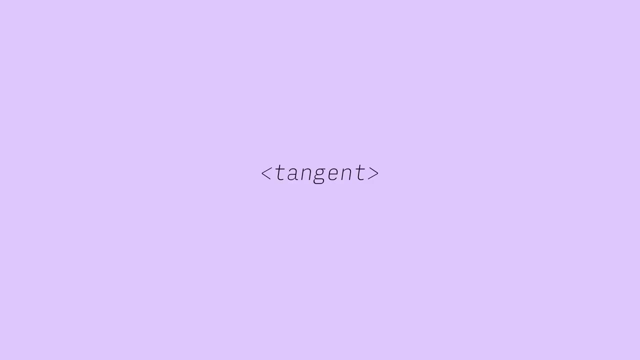 first, no matter where you write it. So quick, tangent. This is basically pretty similar to the difference between imperative and declarative programming. It's commonly explained as telling the computer what to do versus how to do it. For example, if you want to print out a list of 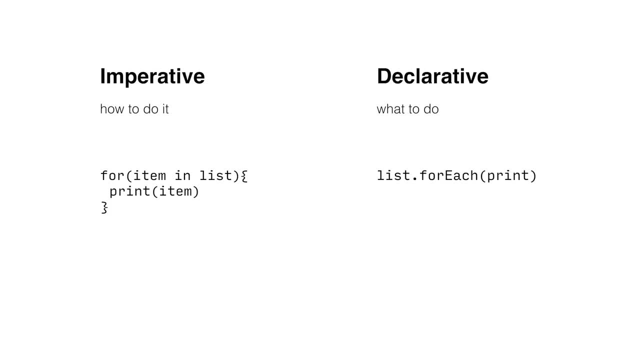 numbers. the imperative way is with a for loop and the declarative way is called dot for each. I found this kind of vague because couldn't you just say I declare for the computer to do a for loop? So the most important part that actually distinguishes between the two is that you don't 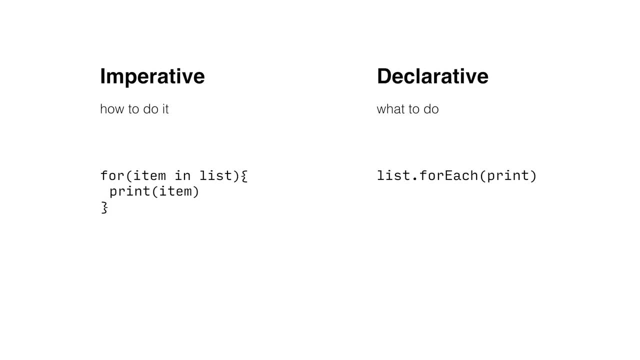 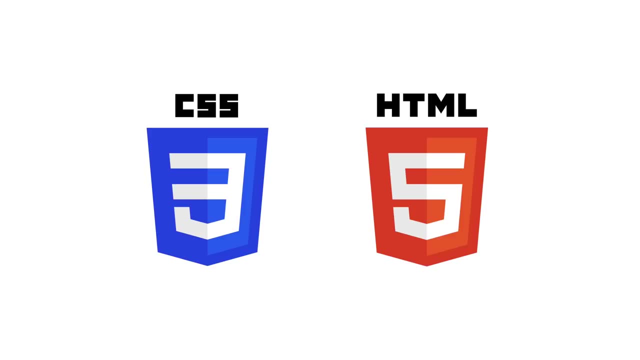 have any manually defined order in the declarative case. But not all declarative things are functional. programming though CSS HTML are declarative because it tells you the layout or the style things should be, but it's not a programming language, but it's still declarative. 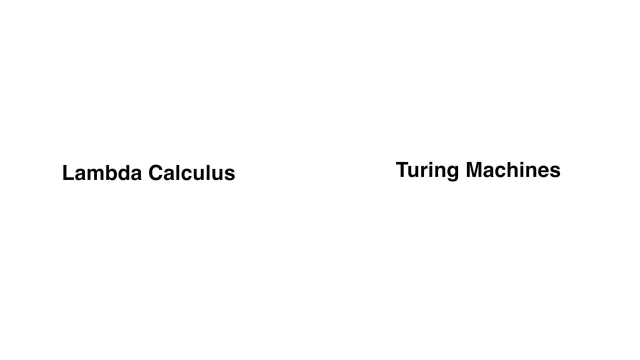 Anyway, however different they are, Alonzo Church and Alan Turing co-published a paper that proved both of them can do exactly the same thing. That means that while Haskell is completely different from regular programming languages, it can do everything. All of this is why Haskell seems so weird when you look at it at first. If you don't, 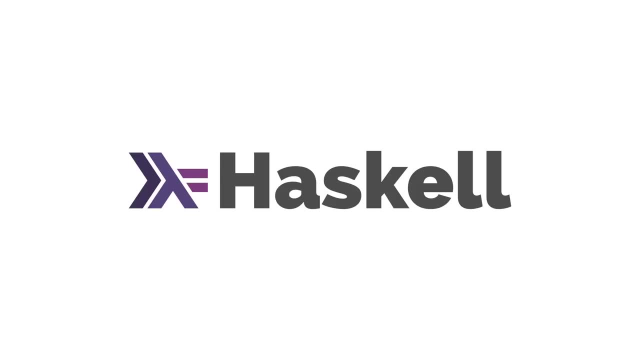 consider the functional programming's mathematical origin, the rules seem pretty arbitrary. Here are the rules the way they're typically said. Functions are pure. This means they have no side effects like printing to the console, changing the file, etc. This weird restriction makes perfect sense if it's like math functions. 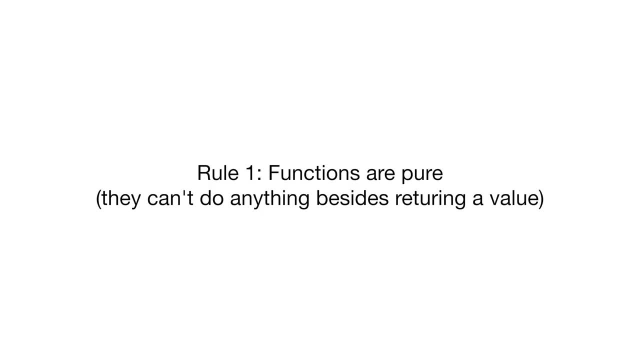 where you take an input and calculate an output, There's no ability to change anything else. So if you want to do things like changing your file, the basic simple explanation is that you can just return a string or return a number and let some other part of the computer handle. 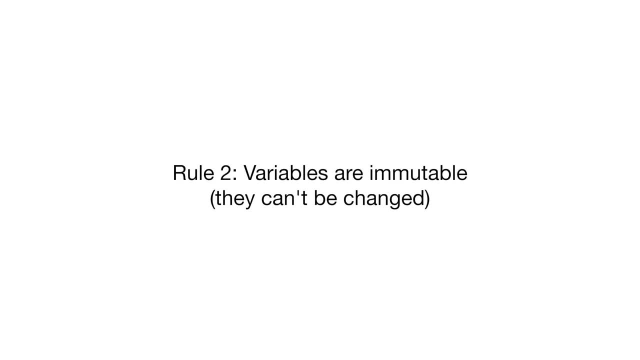 what it does with that. The second rule is that all variables are constants. The common explanation is that making your variables constant makes sense that you won't accidentally change them, which causes problems if other parts of the code is also using it. But it isn't just the organisation trick, It's one of the fundamental 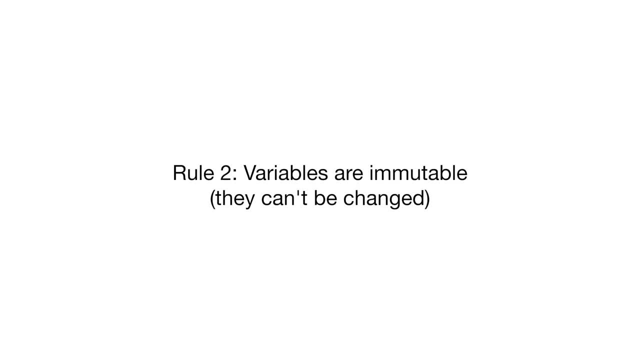 ideas of how functional programming and lambda calculus works. But when we were doing calculations that way, variables had shortcuts for labeling an expression and obviously they wouldn't change. And if you think about it, pure functions can only take inputs and return outputs. there's 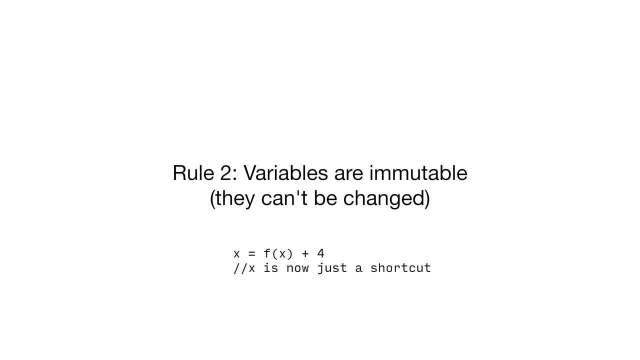 no operation or command to tell the computer to change a variable, so you can't do that at all. As a benefit, the equal sign actually does mean what it means in math and we don't have the confusing x equals to x plus 1 type of thing. 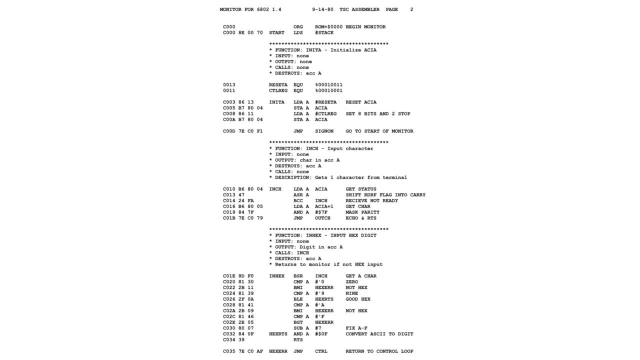 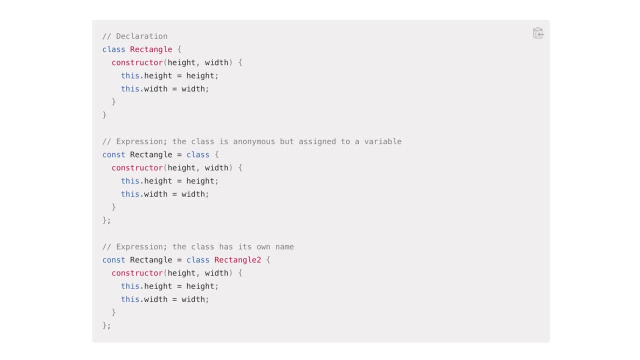 Now as a conclusion, just like how modern computers are more complicated than Turing machines, because Turing machines are meant to just be a simple theoretical example. now we have object-oriented programming, inheritance and blah, blah blah. that isn't part of the construction of a Turing machine. 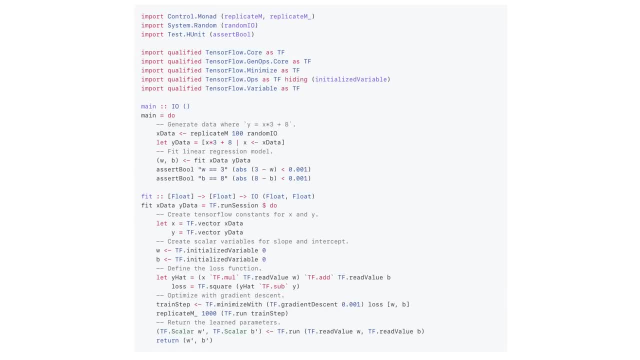 Functional programming, likewise, is also much more complicated than just lambda calculus. But functional rules are a bit more strict. so we can't just tack on another part of syntax, like JavaScript does every other year, and we still have to stick with pure functions. 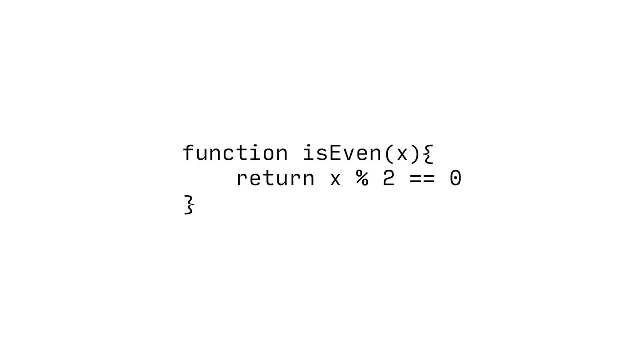 to do everything. So when thinking about making more complicated structures, we think of functions as one-way connections between functions, And it gets interesting when functions themselves are values and you can pass functions into functions. Stuff like that seems to get very messy, but only if you don't know what you're doing. 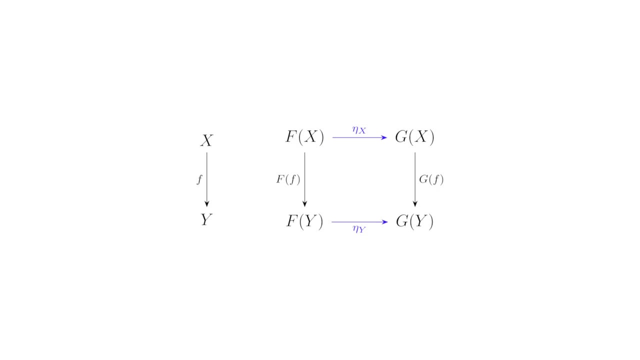 and luckily some people do know what they're doing and have figured out some really fun ways of arranging functions to do really cool stuff. And of course that's another field of mathematics. so make sure to watch the next couple videos in the playlist, where I will go into more depth about lambda calculus.